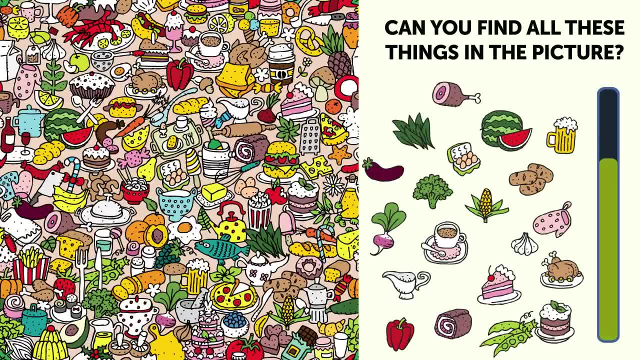 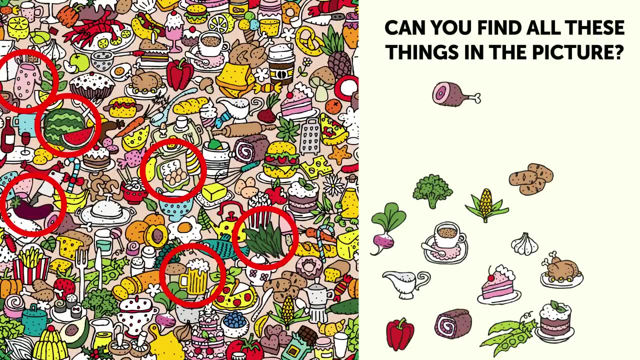 Did you manage to find them all? Here's proof: they really were there. Those peas were pretty hard to find, don't you think? Number three, I'll give you 10 seconds to tell which glass has more water in it. If you have a paperclip, eraser and watch are in there for a reason. 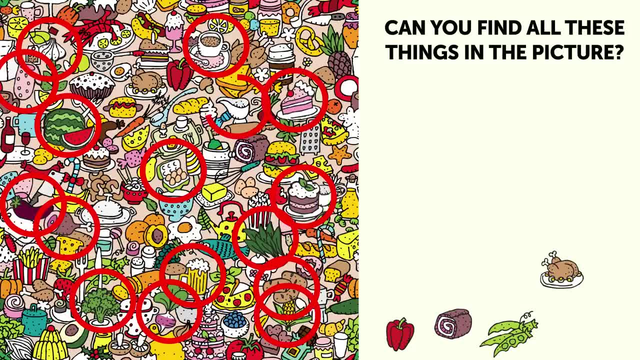 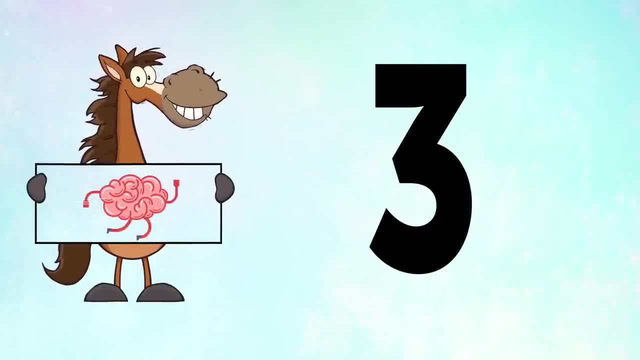 The answer is B- The paperclip has more water in it. So I'll explain why. Number three: What figure should replace the question mark? You've got 10 seconds to figure it out. The answer is B- The iron has more water in it. So if you have a paperclip, eraser and watch are in there for a reason. 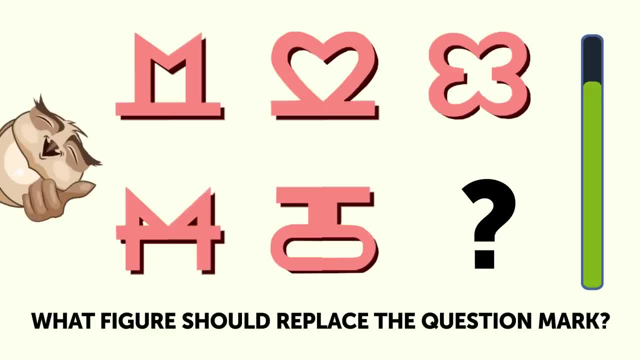 The answer is C: If you have a paperclip eraser and watch are in there for a reason. If you have a paperclip eraser and watch are in there for a reason. So if you have a paperclip eraser and watch are in there for a reason, 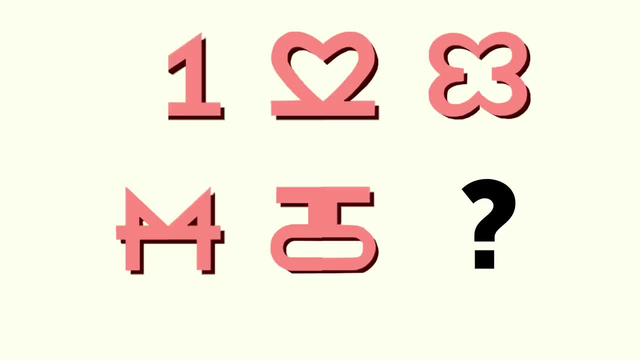 Here's proof. they really were there for a reason. Either that or you can just use a ruler, So just think about it. It's important to know that the paperclip is water. So did you manage to see the hidden pattern in these weird shapes? 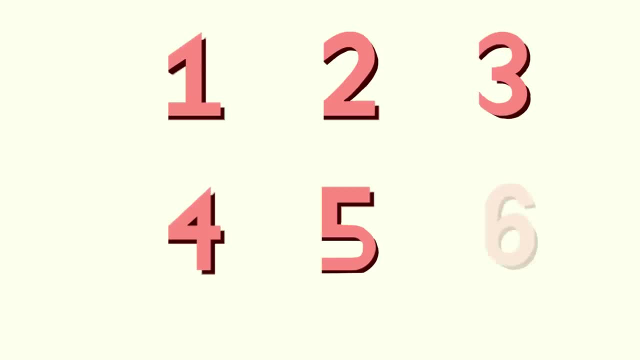 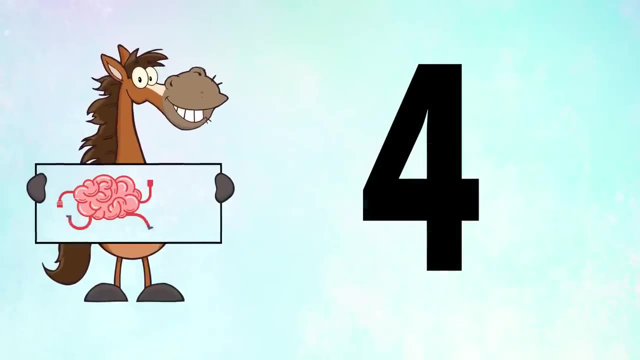 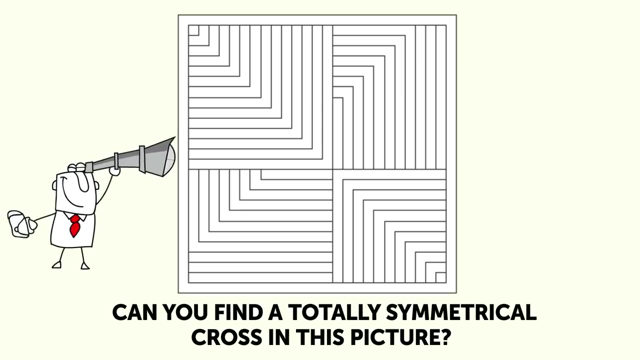 They are all numbers with their mirrored reflections to the left. So the right answer here is a 6 and its backwards twin, Number 4.. Can you find a totally symmetrical cross in this picture? You have 10 seconds to read between the lines. 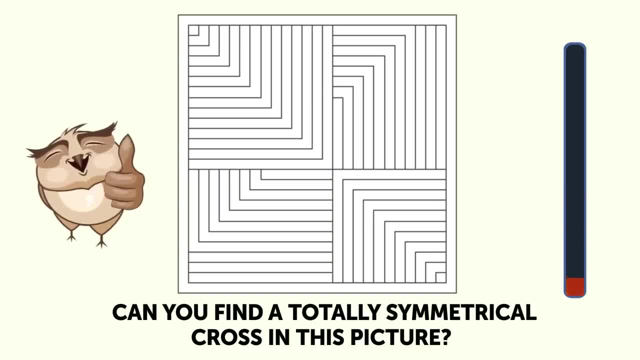 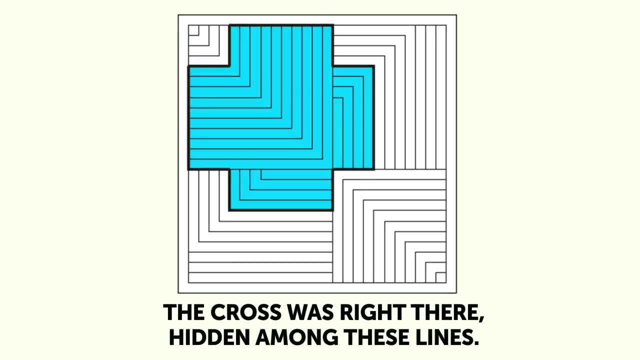 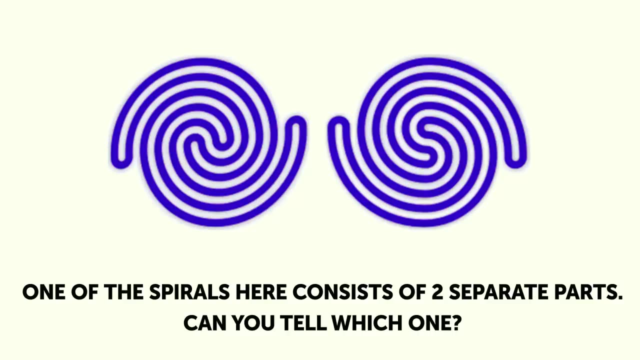 Oh, there you go. The cross was right there, hidden among these lines, Number 5.. Try not to get hypnotized by this next riddle. One of the spirals here consists of two separate parts. Can you tell which one? 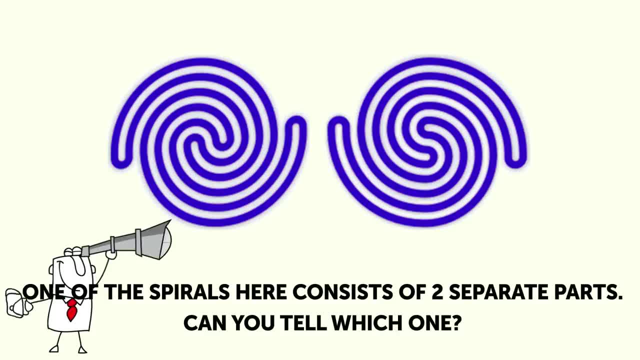 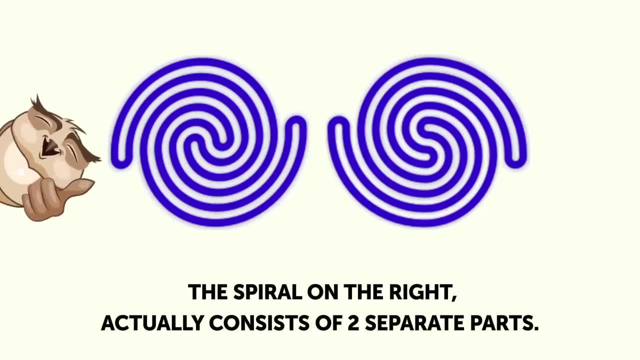 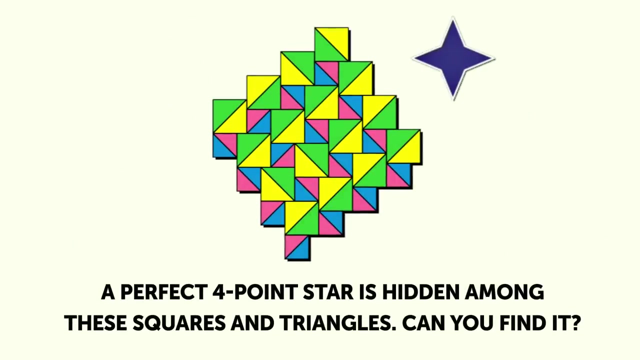 You know the drill, 10 seconds on the clock. The spiral on the right. even though it looks pretty much identical to the left, one actually consists of two separate parts. Number 6. A perfect four-point star, like the one right here. 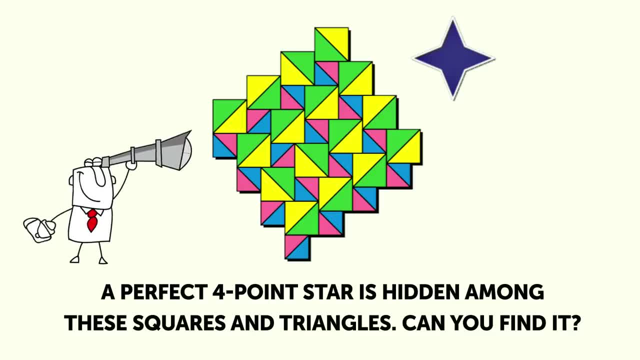 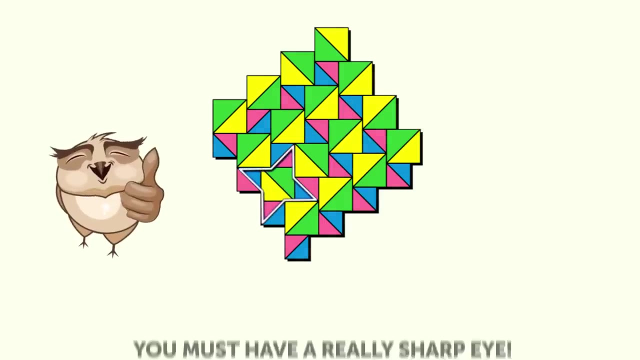 is hidden among these squares and triangles. Can you find it? Your time starts now. Ah, that was a tricky one, wasn't it? The star was right down there all along. Hit the thumbs up if you managed to find it. You must have a really sharp eye. 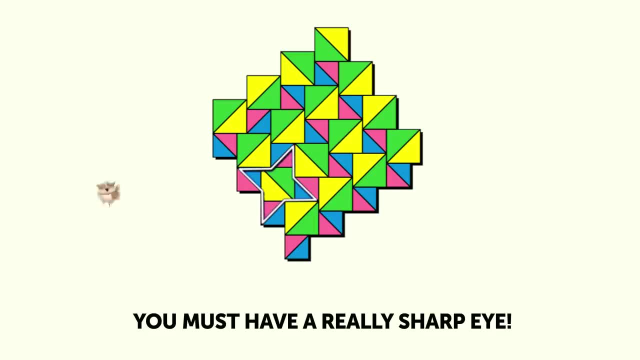 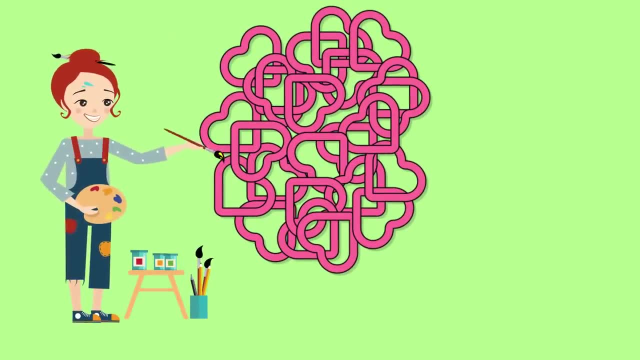 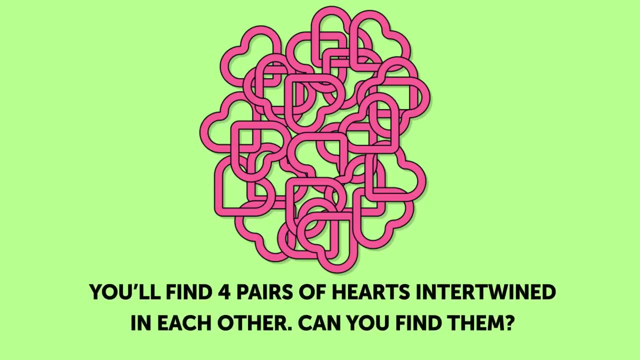 Ow, Maybe too sharp. Uh, can you get me a band-aid Number 7.. This picture might just look like a teenage girl's messy arts and crafts project, But if you look closely you'll find four pairs of hearts intertwined in each other. 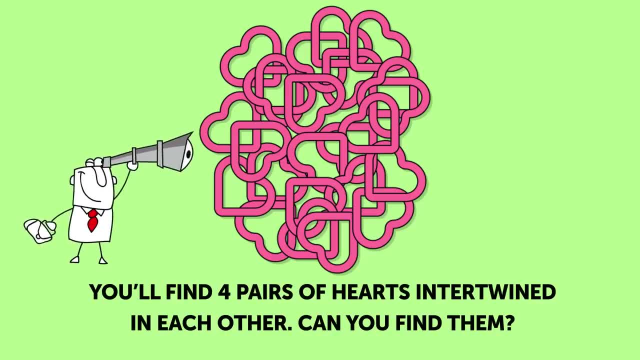 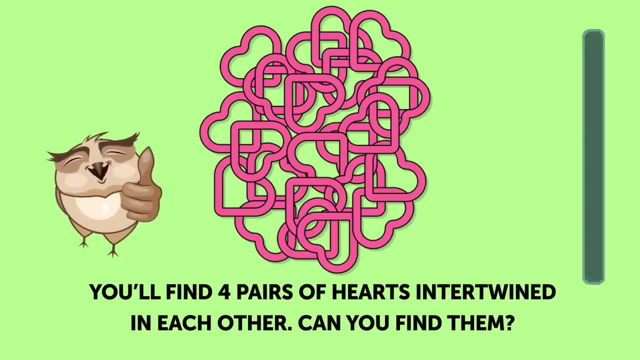 Ha-ha-ha-ha, Ha-ha-ha-ha, Ha-ha-ha-ha, Ha-ha-ha-ha, Ha-ha-ha-ha, Ha-ha-ha-ha. Some hearts are forever bound together. 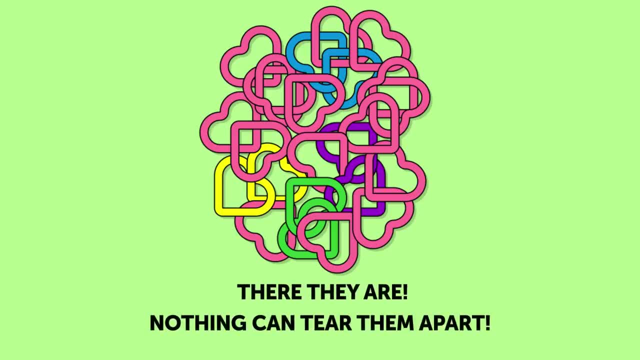 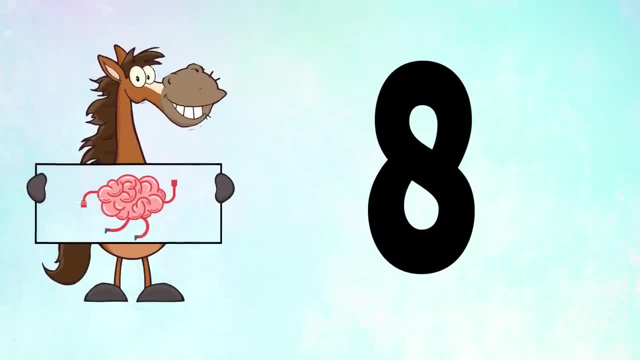 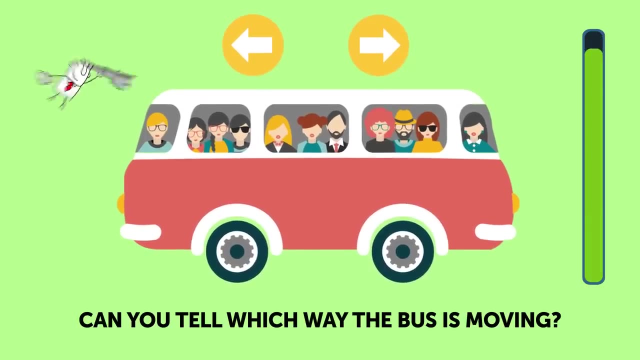 That's definitely the case in this picture. There they are. Nothing can tear them apart. Number 8.. Time for a little road trip. Can you tell which way the bus is moving? Ha-ha-ha-ha, Ha-ha-ha-ha. 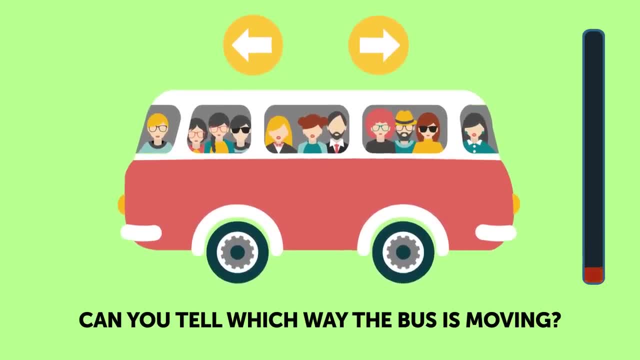 Ha-ha-ha-ha, Ha-ha-ha-ha. So if you're trying to find the driver or carefully examine the passengers, nice try, But it's way simpler than that. Bus doors are always on the right side. 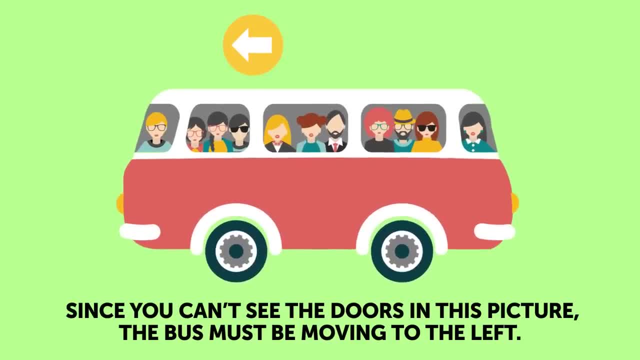 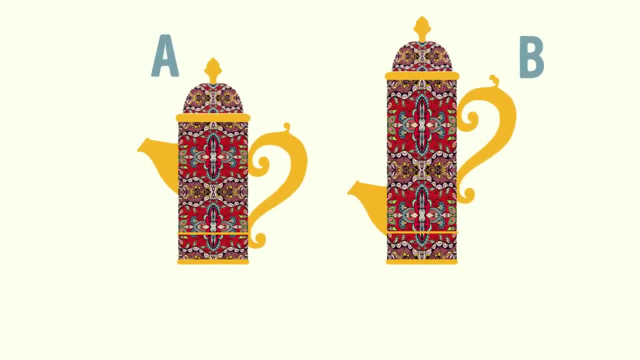 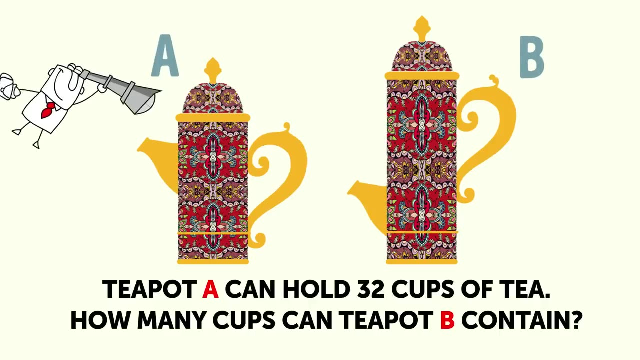 Since you can't see the doors in this picture, the bus must be moving to the left- Number 9.. How about we finish this brain workout with some tea? Teapot A can hold 32 cups of tea. How many cups can teapot B contain?